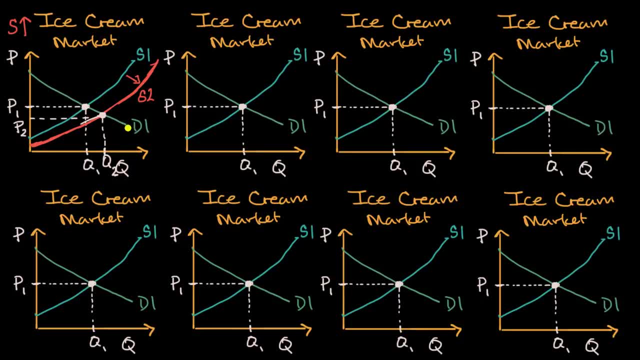 Once again, assuming that we have a downward sloping demand curve like this, which is what you would typically see, And so in this case, let me just write it here- We have our quantity, or actually, let me write it this way: 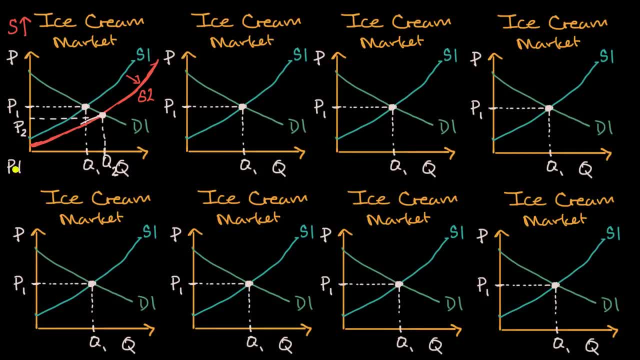 We have: our price goes down and our quantity goes up. Alright, now let's do this example and let's imagine the other way. Let's imagine in this scenario, our supply goes down. What is going to happen to this graph? 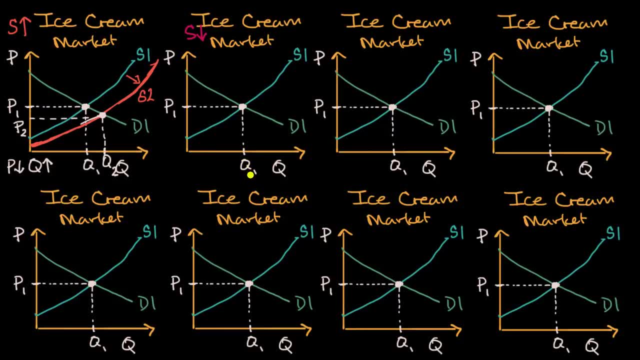 And, in particular, what's going to happen to our equilibrium price and our equilibrium quantity. Well, in this situation, for a given price, people are willing to supply less. That's how I like to think about it. So we would have a shift to the left and up. 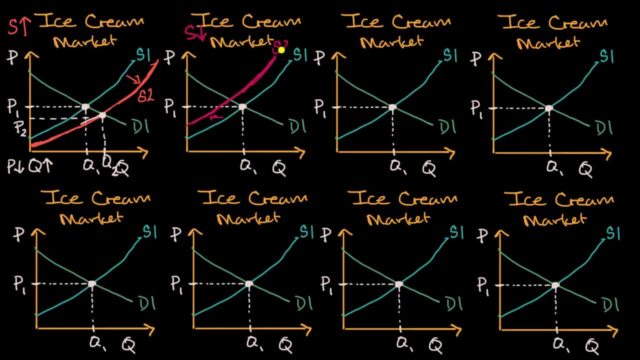 And so we could call this supply curve 2 right over here. And then what is our equilibrium point? It's right over there, It is right over there, And so this would be our new price. It has gone up, And this would be our new quantity. 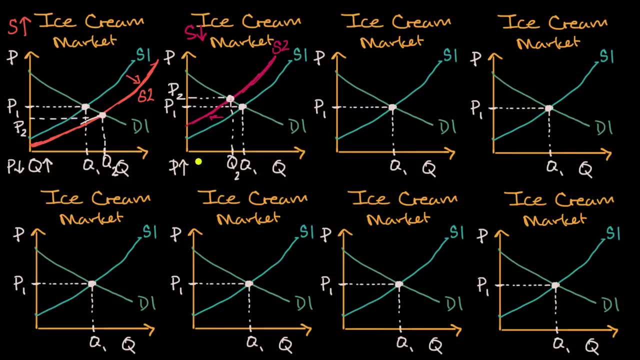 It has gone down, So price has gone up And quantity has gone down. And once again, in either of these scenarios- hopefully, this feels a little bit like common sense- If you have a supplier enter into the market, there's going to be quantity might go up. 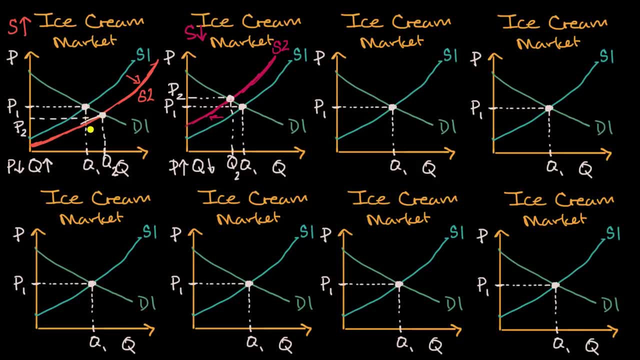 and there's more competition amongst the suppliers, And so the price would go down Here, where the supply goes down, maybe some of the ice cream stores close down. Well now the quantity will go down, There's just less people supplying. 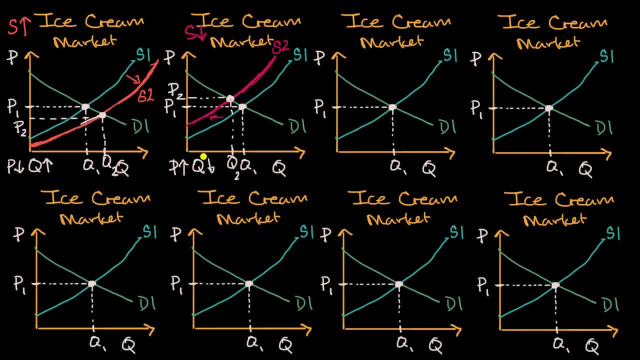 But the price goes up For the ice cream. that's there. the equilibrium price is going to be higher. Now let's do the same thing with the demand curve. Let's think about a situation where- first, let's think about a scenario where- demand goes up. 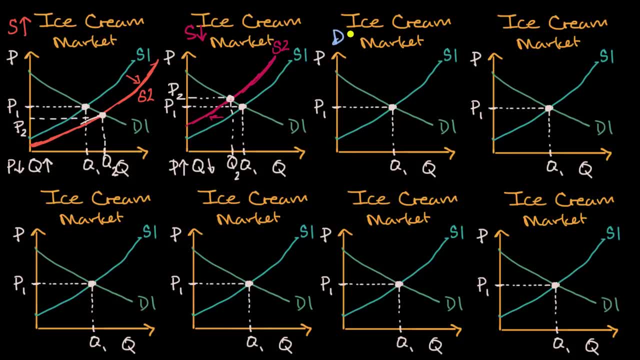 Demand goes up. What is going to happen in this world? Well, demand might go up because maybe there's some type of report that ice cream is much healthier for you than expected, And so, at a given price, people are willing to demand a higher quantity. 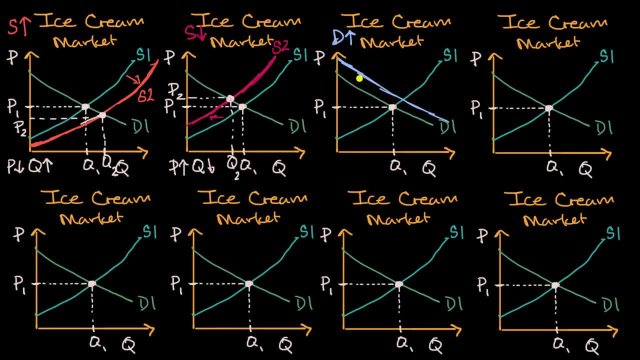 So, for example, at that price, people would demand a higher quantity, And so we would have a shift to the right and up- Let's call this D2 right over here, And this is our new equilibrium point, And then notice what has just happened here. 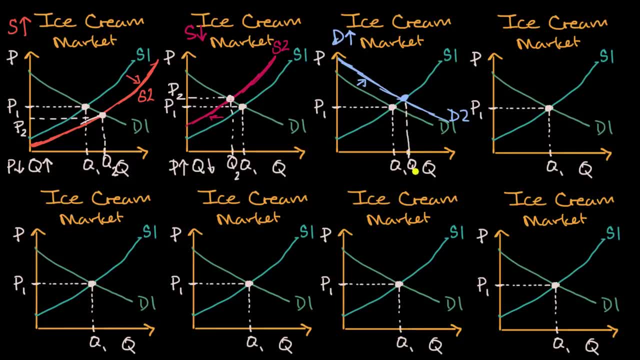 At our new equilibrium point. this is Q2, and then this right over here is this right over here is P2, our new price, our new equilibrium price and our new equilibrium quantity. In this situation where demand goes up, both price and quantity are going to go up. 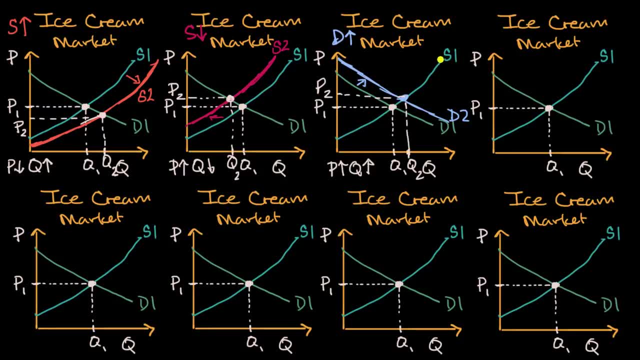 assuming we have this upward sloping supply curve again, And once again that makes sense. More people just want to buy ice cream. The supply curve dynamics have not changed, so we're going to move along that supply curve to the right and up. 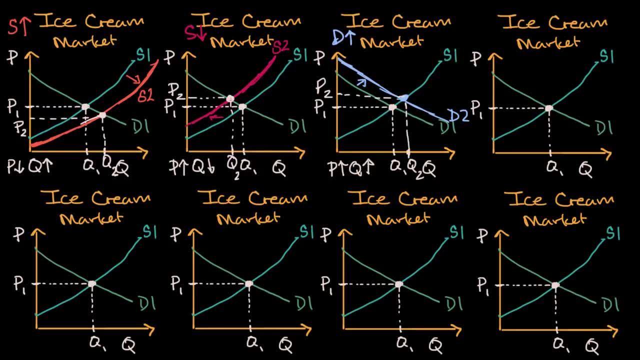 So both price and quantity go up. Well, if demand goes down, you can imagine the opposite is going to happen. So here, if we have demand goes down, let's say a big study comes out that ice cream is even unhealthier than we originally thought. 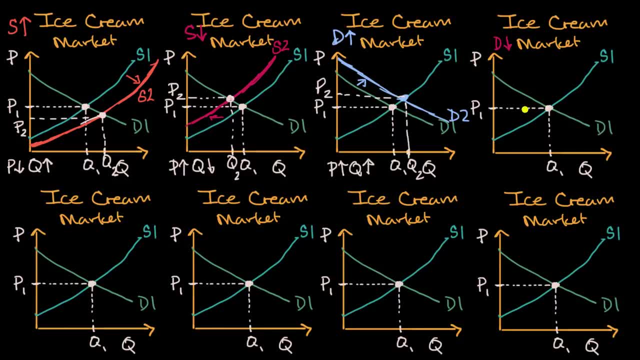 well then, at a given price, people are going to want, they're going to demand- less ice cream, And so our demand curve would shift to the left and down. So we'll call this D2 right over here, And then we can see our equilibrium: price and quantity. 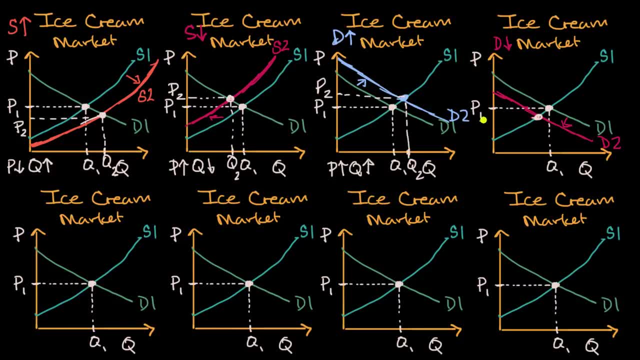 So let's show that new equilibrium price is P2 right over here, And then our new equilibrium quantity is Q2.. And notice, both price and quantity go down. People just don't want to buy ice cream as much because they think it's unhealthy. now 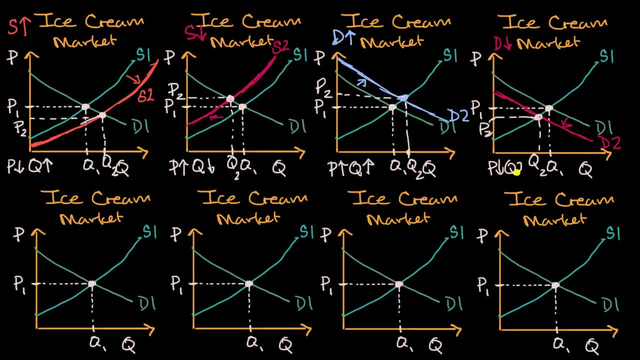 So price goes down and quantity goes down.